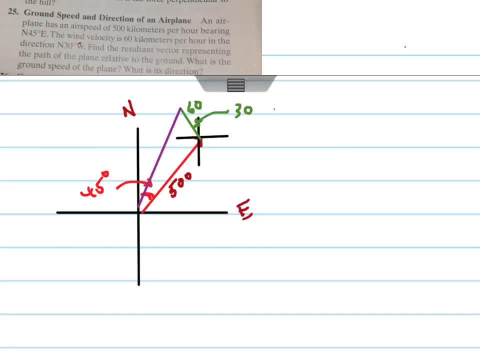 Oops, that wasn't good. Still not good. Alright, So let's take a look at all of our different angles that we have here. Alright, so what we have is an oblique triangle, And so we're going to use either the law of sines or the law of angles. 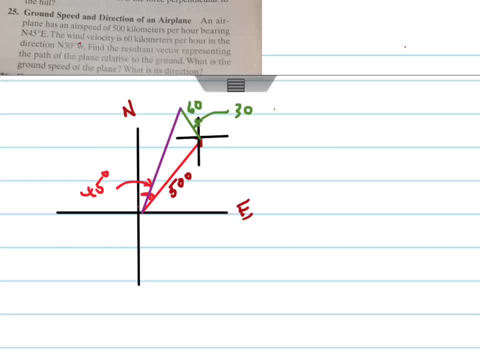 And so we're going to use either the law of sines or the law of cosines, based upon what we had. and you'll notice here that this angle inside, right here, right there, is 60 degrees, so that angle gets kind of tighten. here is 60 degrees. 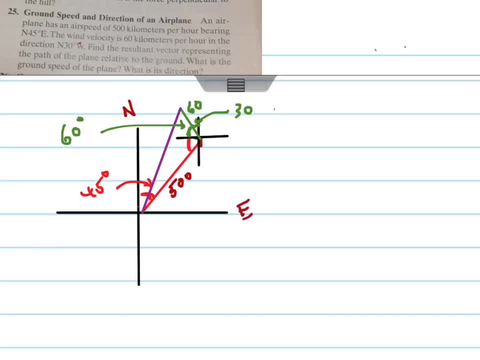 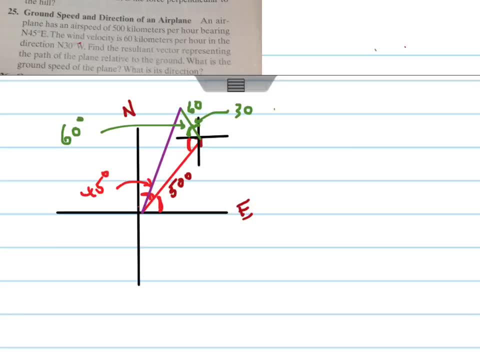 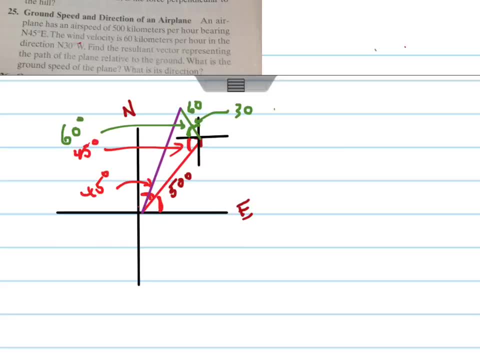 total angle: right, there is 105 degrees, So let me pull that triangle out. There's the angle that the purple line. I'll do the color coding here so it's easier to see. There's the green line and the red line would look something like that And this angle right. 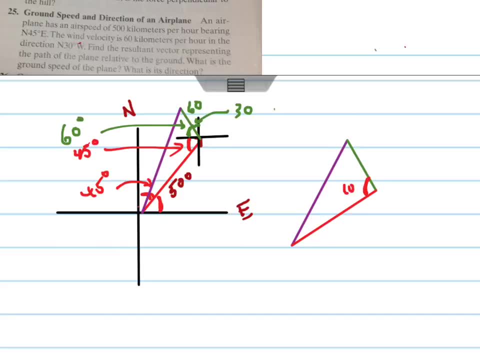 here is 105 degrees, This side is 60, and this side is 500, and so the law of cosines was going to allow me to find the length of that purple side. 007 is the distance that I want to find, and the law of cosines is, if you remember correctly, 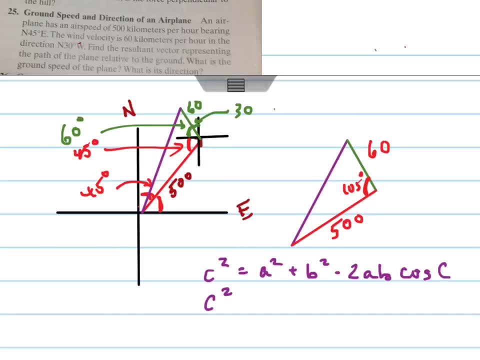 there's your law of cosines. so we have: c squared equals 60 squared, plus 500 squared, minus 2 times 60 times 500 times the cosine of 105 degrees, and when I solve that I would get you will get 518.78 kilometers per hour. so that's this right here: 518.78,.